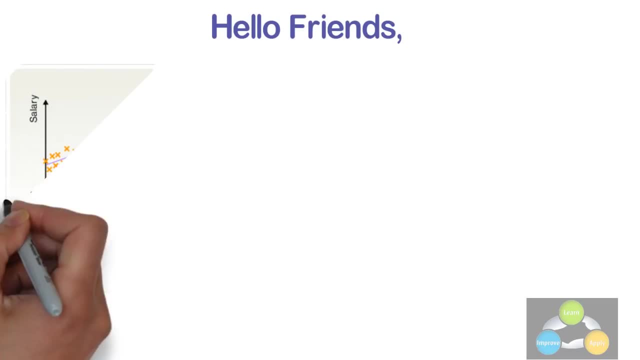 Hello friends, in the last video of scatterplot we had seen how to detect relationship between two or more variables by using scatterplot and looking at the trend of scatterplot. But only obvious relationships can be detected easily by looking at the graph. In some cases, 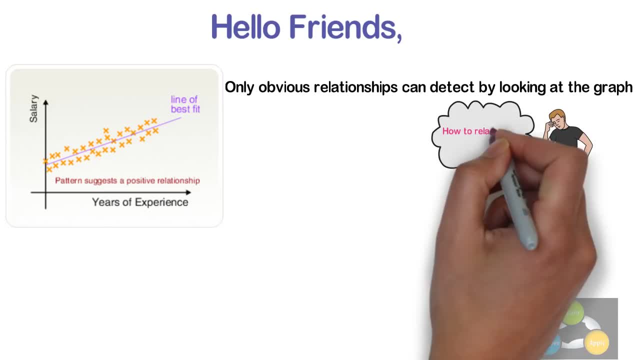 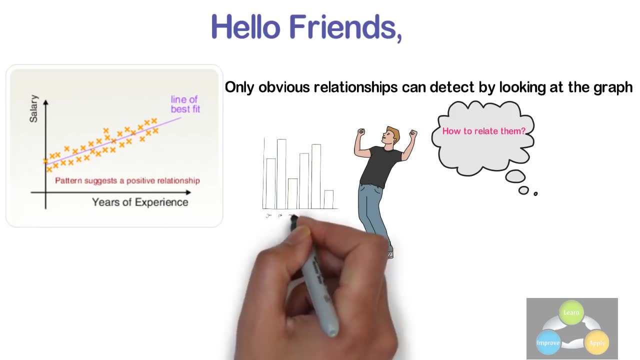 it is not possible to judge the relationship between two variables only looking at the graph, But the good thing is that we can comment about the relationship between these variables using statistics. Yes, I am going to explain the use of statistics in determination of relationship between these variables, as well as to predict the response of one variable. 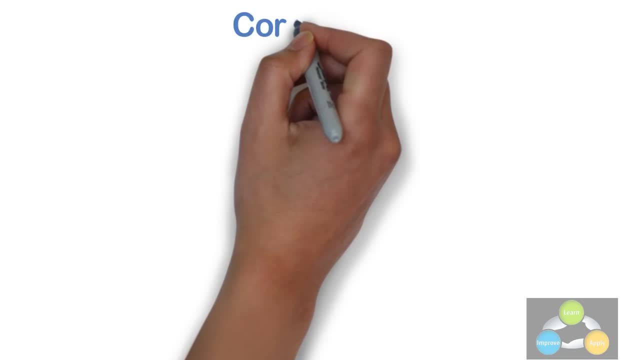 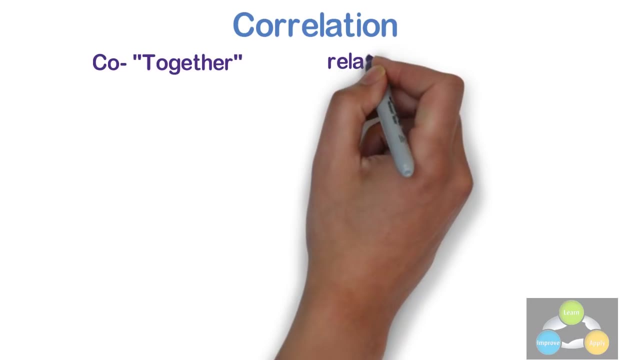 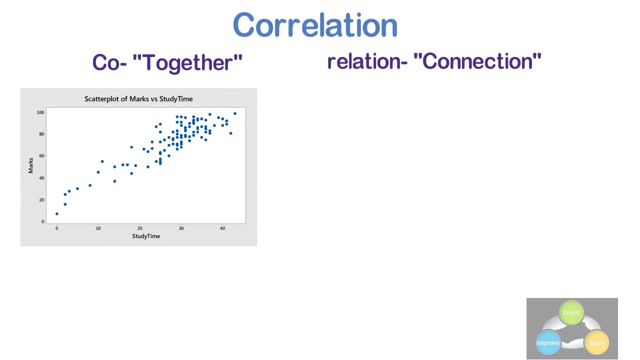 if we know the value of another variable. So let's begin Correlation. The term correlation is a combination of two words: Co means together, and relation means connection between the two quantities. Correlation is when, at the time of study of two variables, a unit change in one variable is realized. 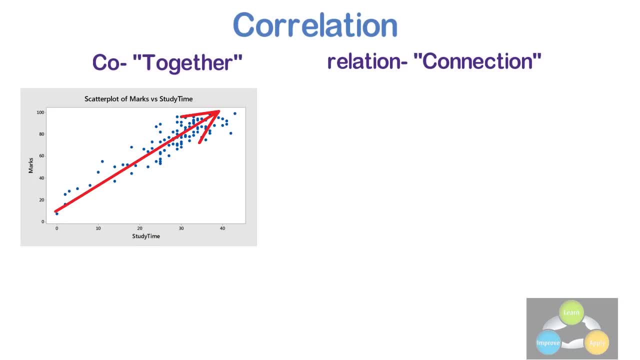 by an equivalent change in another variable, directly or indirectly, Or else the variables are said to be uncorrelated when the movement in one variable does not show any movement in another variable in a specific direction. It is a statistical technique which represents the strength of connection between the layers of variables. Correlation can be positive. 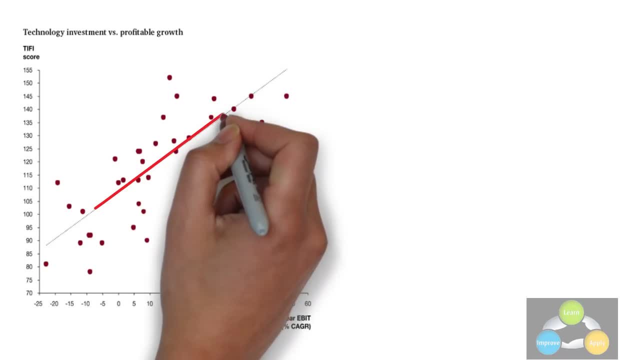 or negative When the two variables move in the same direction. that is, an increase in one variable varies from one variable to another variable. Correlation can be positive or negative, result in corresponding increase in another variable and vice versa. then the variables: 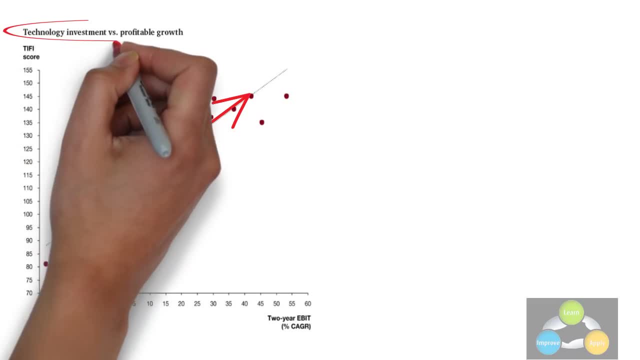 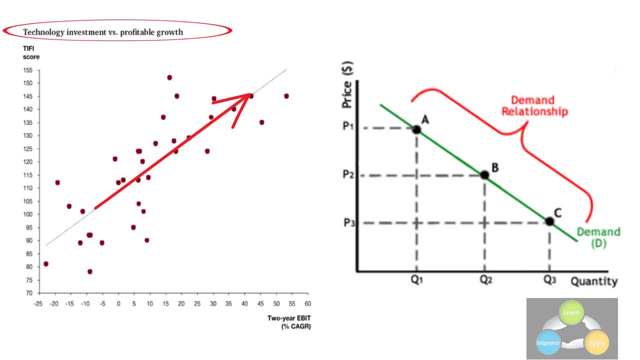 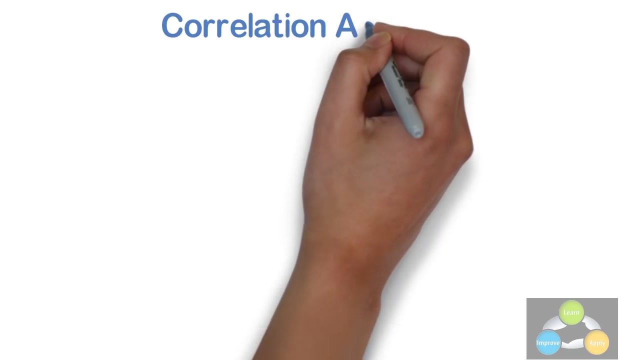 are considered to be positively correlated, for example, profit and investment. On the contrary, when the two variables move in the different direction in such a way that an increase in one variable will result in decrease in another variable, and vice versa, this situation is known as negative correlation. for example, price and demand of a product. 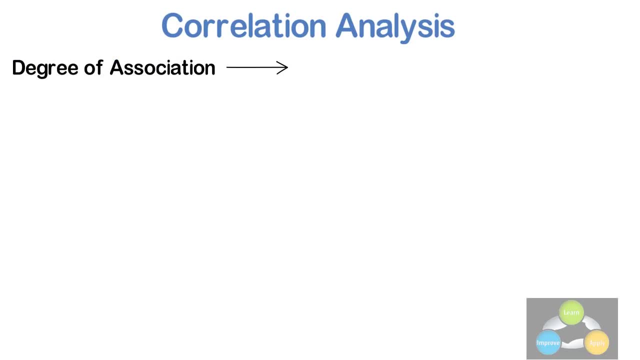 Correlation Analysis. The degree of association is measured by a correlation coefficient denoted by R. It is sometimes called as Pearson's correlation coefficient, after its originator and is a measure of linear association If a curved line is needed to express the relationship. other and more complicated measures of correlation. 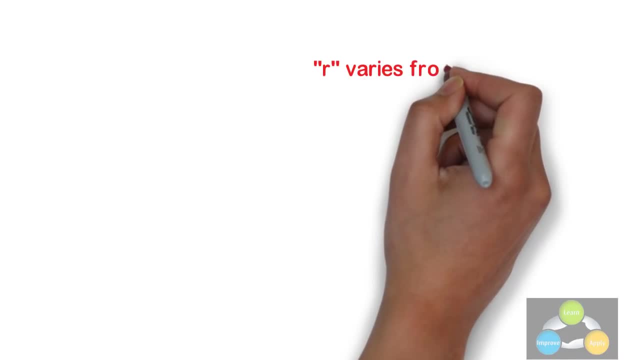 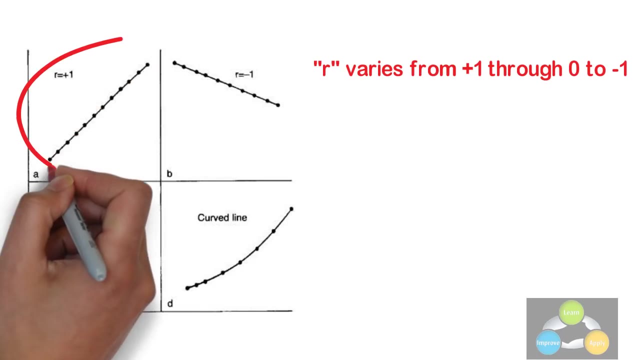 must be used. The correlation coefficient is measured on a scale that varies from plus one through zero to minus one. Complete correlation between two variables is expressed by either plus one or minus one. When one variable increases as the other increases, the correlation is positive. When one decreases as the other increases, it is. 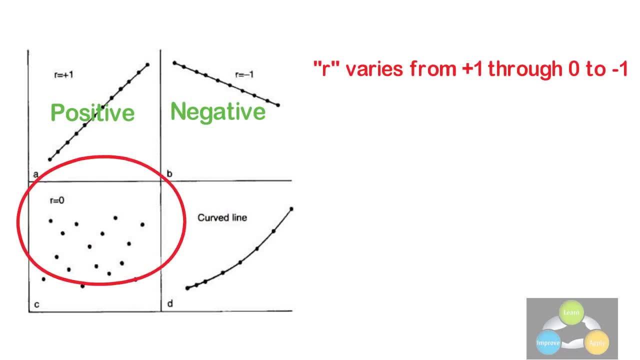 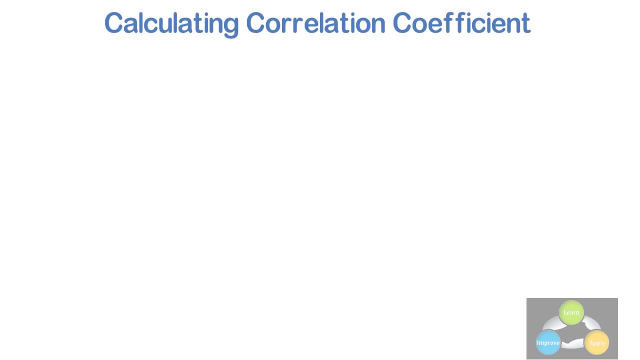 negative. Complete absence of correlation is represented by zero. This figure gives the some graphical representations of correlation. Calculating Correlation Coefficient. This coefficient is easily calculated by using Microsoft Excel and Minitab. Correlation Coefficient by Excel. There are two simple methods to calculate. 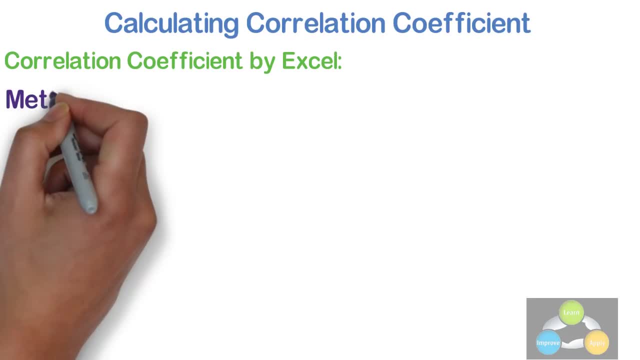 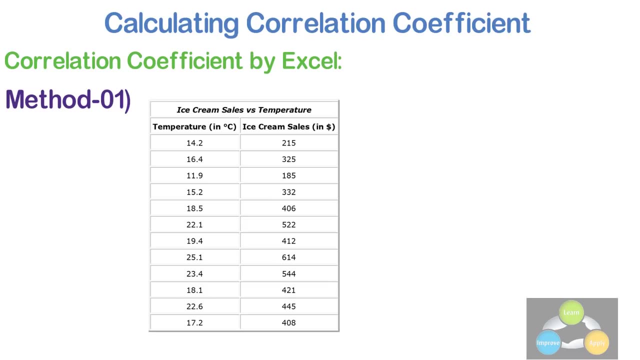 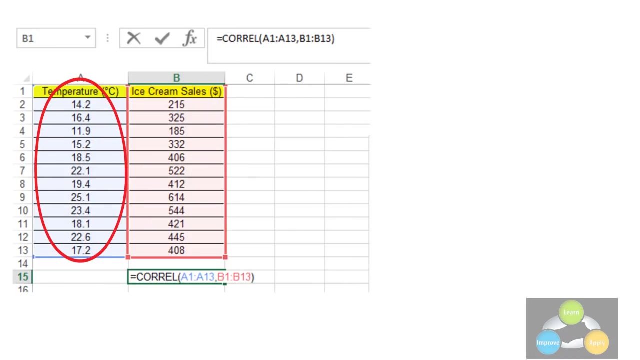 the correlation coefficient in Excel Method 1. Let's take an example of temperature of the day versus ice cream sale. To determine the correlation between these two variables, use a function CORREL, Type the function CORREL and select first variable column and apply comma. After that select second variable column. 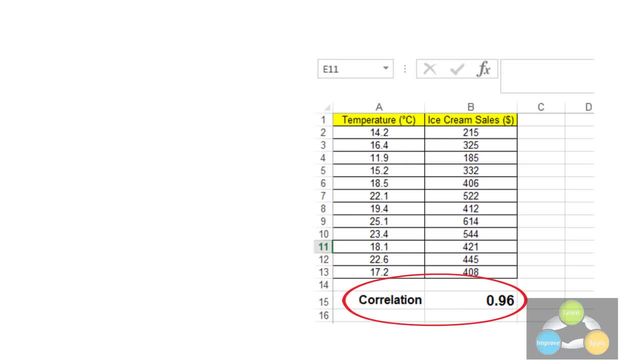 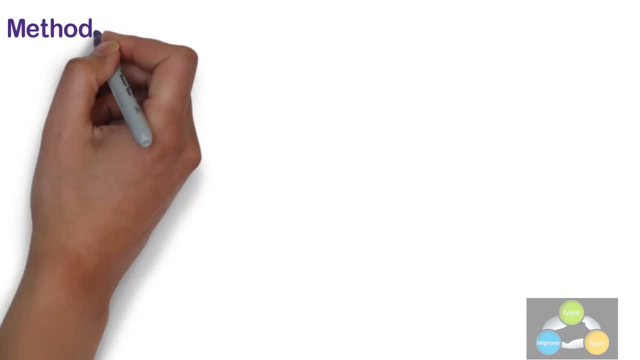 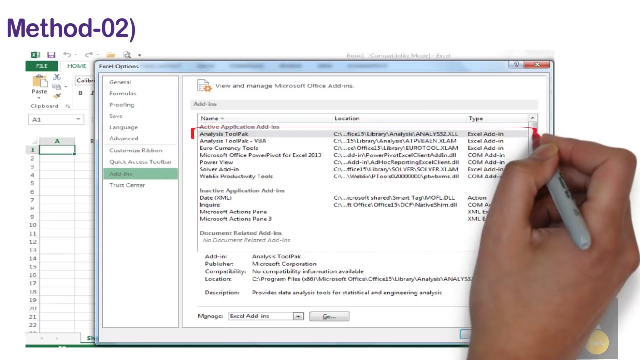 and press enter, We will get the value of correlation coefficient as 0.96.. It means there is a strong relationship between variables. Method 2: Let's continue with the same example. To determine relationship between these two variables, use the analysis tool pack add-in in Excel to quickly generate the correlation. 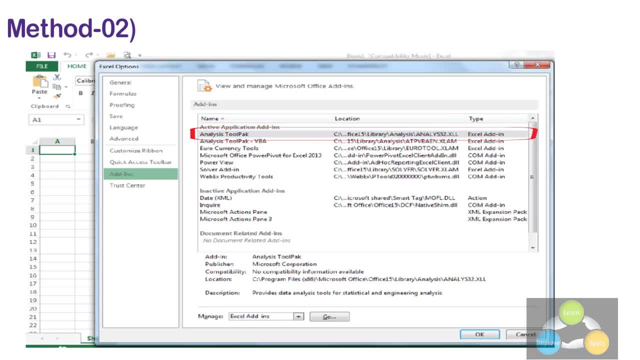 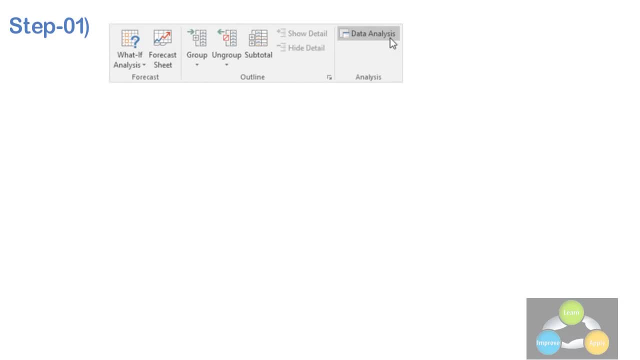 coefficients between multiple variables, We need to execute the following steps: Step 1.: 1., 2., 3., 4., 5., 6., 7., 8., 9., 10., 11., 12.. 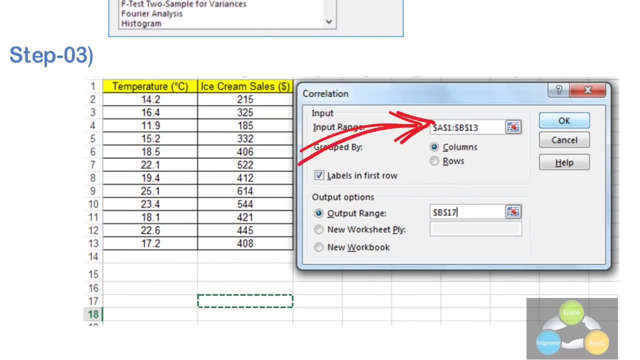 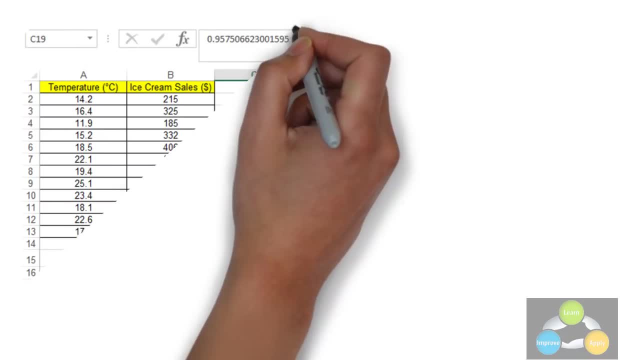 12., 13., 14., 15., 16., 17., 18., 19., 20., 21., 22., 23., 24., 25., 26., 27., 28.. 29., 30., 31., 22., 24., 25., 26., 26., 27., 27., 28., 29., 29., 30., 31., 32., 32.. 33., 34., 35., 36., 37., 38., 38., 39., 39., 40., 41., 42., 42., 43., 44., 45., 46.. 47., 48., 49., 50., 51., 52., 53., 52., 53., 54., 55., 56., 57., 58., 59., 60., 61.. 62., 62., 63., 63., 64., 65., 67., 68., 67., 68., 69., 69., 70., 71., 72., 72., 73.. 73., 74., 74., 75., 76., 77., 78., 78., 79., 79., 80., 80., 81., 82., 82., 83., 83.. 84., 84., 85., 86., 87., 82., 85., 86., 87., 88., 88., 88., 89., 89., 90., 92., 92.. 92., 93., 93., 93., 94., 94., 94., 95., 95., 96., 96., 97., 97., 98., 98., 99., 100.. 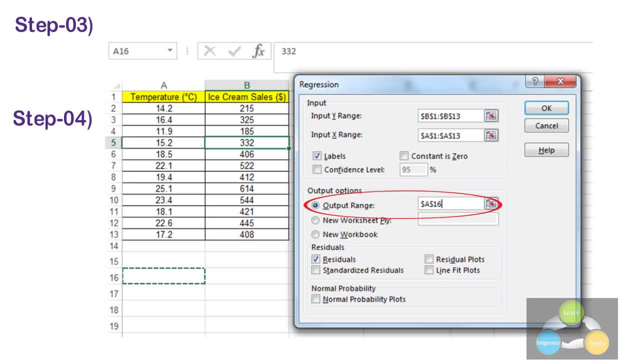 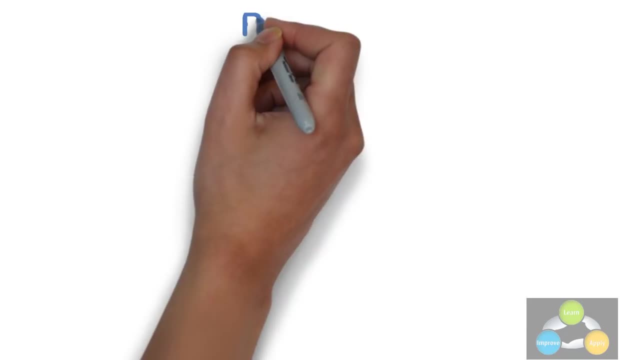 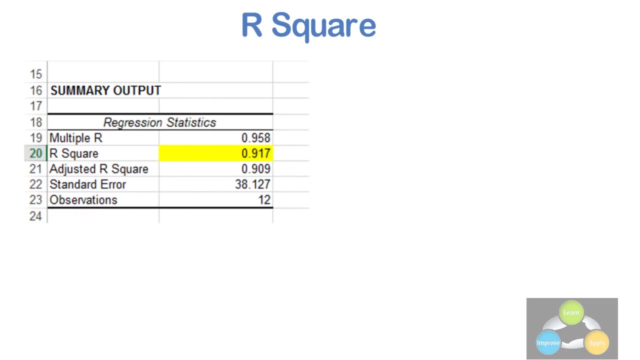 and select cell A16.. You can select anywhere in the sheet as well as in the separate worksheet. Check residual and click OK. Excel produces the following summary output: Rounded it to the three decimal places, R square. R square equals 0.917, which is a very good fit. 92% of the variation in ice cream. 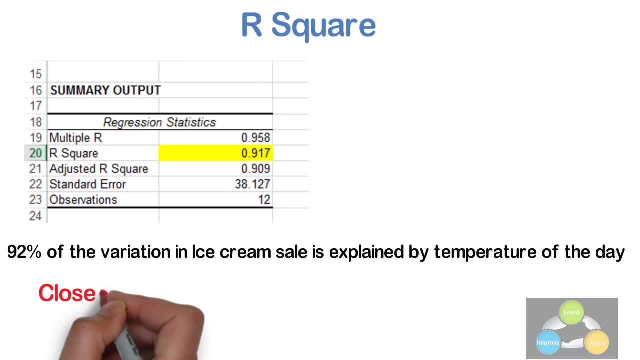 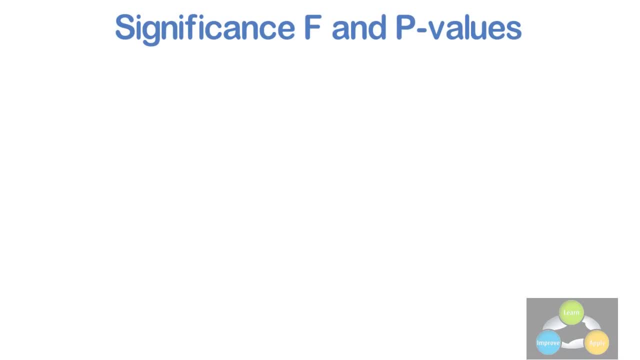 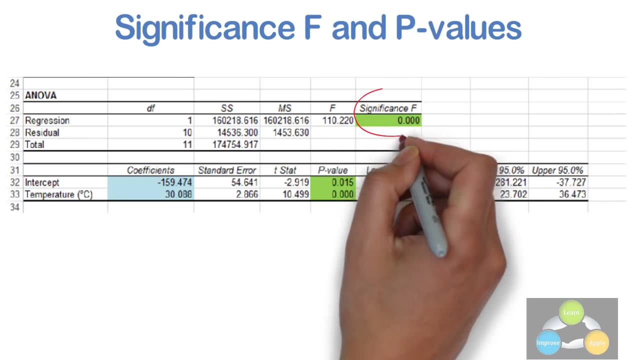 sale is explained by the temperature of the day. The closer to 1, the better. the regression line feeds the data. Now let's see the significance F and P values To check if your results are reliable. that is statistically significant. look at significance F, value 0.000.. If this value is less than 0.05, you are okay. 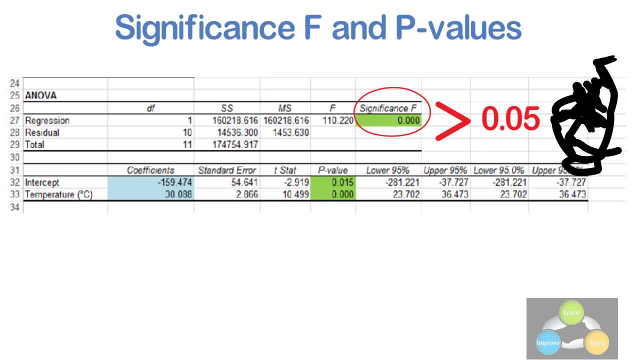 If significance F is greater than 0.05, it's probably better to stop using this set of values. Delete a variable with a high P value that is greater than 0.05 and return the regression until significance F drops below 0.05.. All P values be. 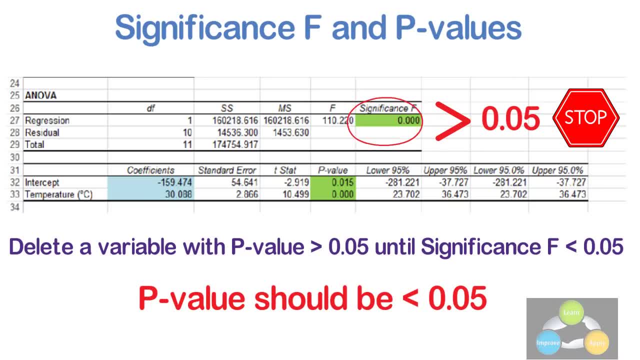 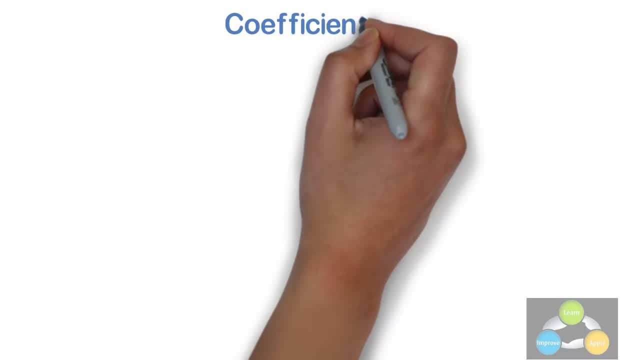 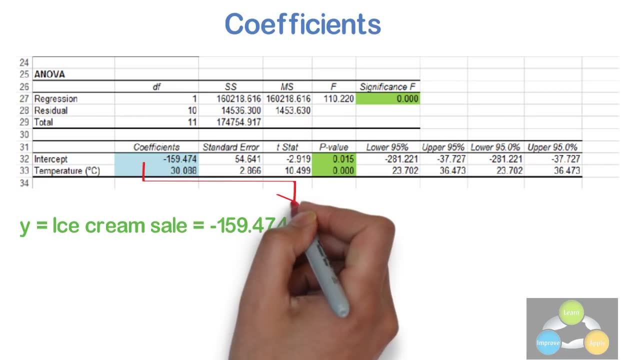 below 0.05.. In our example, this is the case 0.015 and 0.000.. Coefficients: The regression line is: Y is equal to ice cream sale, which is equal to minus 159.4, 74 plus 30.08 into temperature of the day, In other words, for each unit increase. 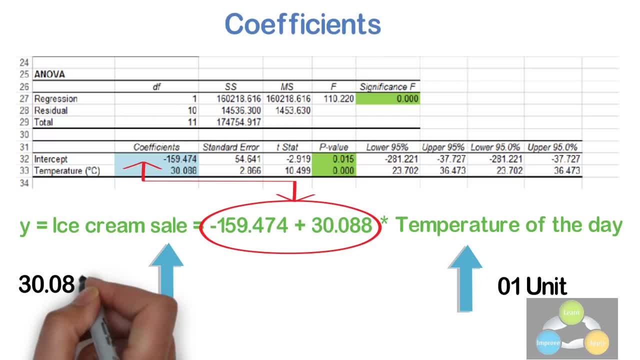 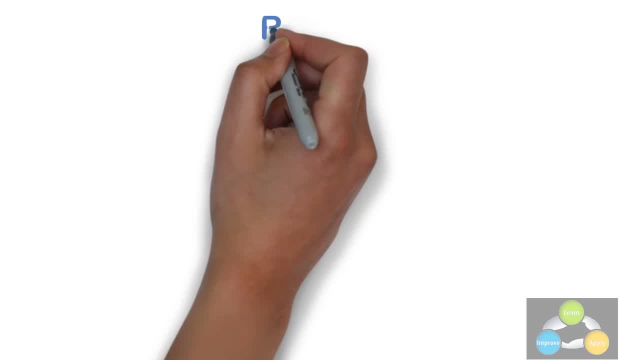 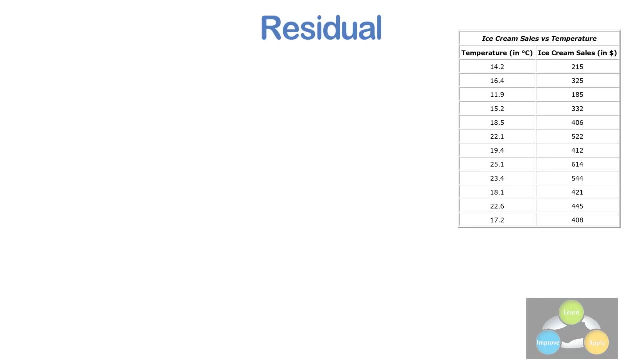 in temperature ice cream sale increases by 30.08 units. This is a valuable information. You can also use this coefficients to do a forecast Residuals. The residuals show you how far away the actual data points are from the predicted data points. using the equation, For example, the first data points equals 2.5.. 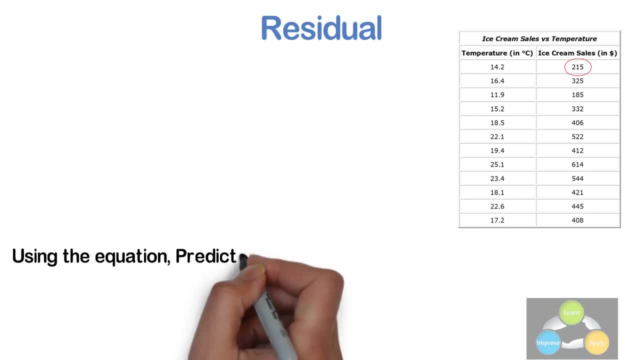 Using this equation, the predicted data points equals minus 159.474 plus 30.088 into 14.2, which is equal to 267.773, giving a residual of 267.773 minus 215, which is equal to minus 52.773.